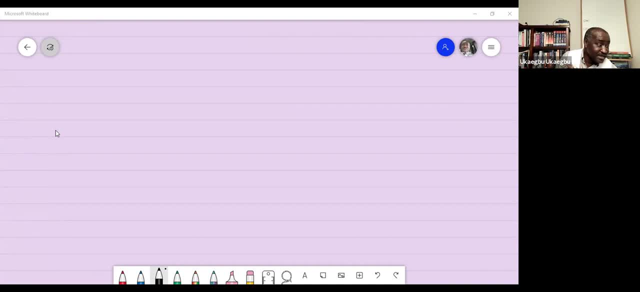 exact same feature that you see on TI-84.. You need it. So you need a graph paper, You need a cell phone, You need a pencil, You need a ruler or something beside you, And we are going to start by writing non-linear systems of equation and solving them graphically. 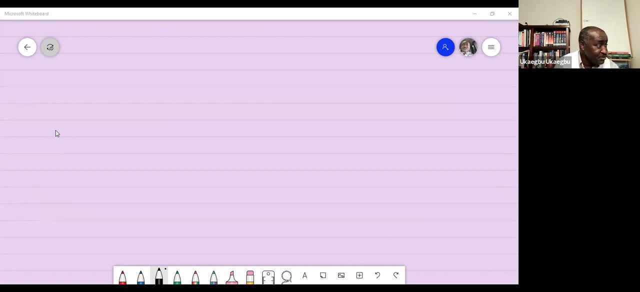 Okay, So if you have your test book, you can make reference to page 472.. You can make reference to that page, But what we are going to do today is hands-on. So you are going to be generating the data and you are going to be plotting the graph. All right, So let me write, you know. 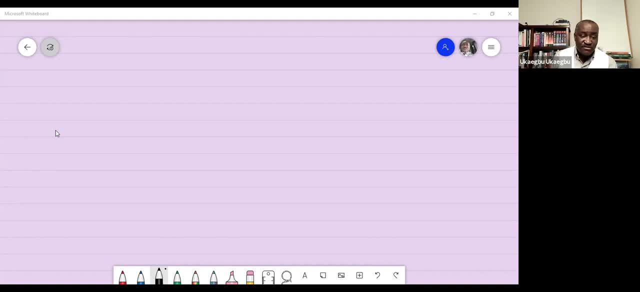 just to get started, let me write a system of non-linear equation And we shall use graphical method to solve it. Okay So let me write the topic. What page did you say, Mr Gregoire? Yeah, you can make reference to page 472.. Okay So, once again, the topic is graphical method. 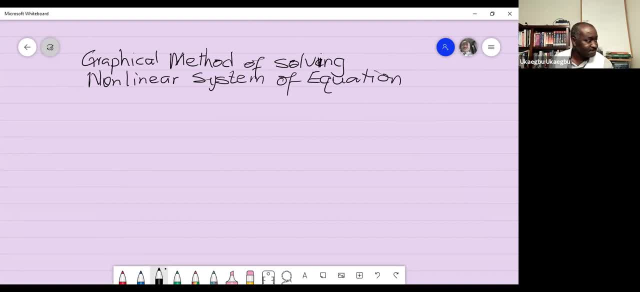 of solving non-linear system of equation. The question once again is: why do we have to do this? We have to do it because Because non-linear system of equation has a lot of application in the real world And because of that it falls into the curriculum of high school mathematics. Press Pre-calculus. 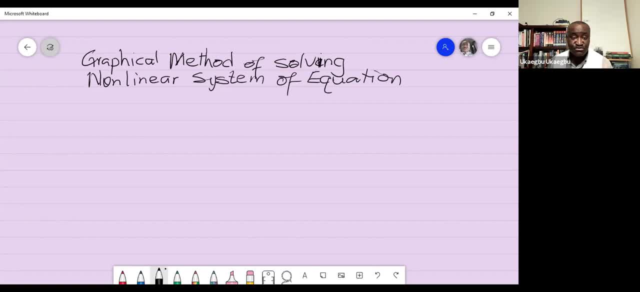 precisely for us to figure out how to solve these non-linear systems of equation using graphical method. Okay, So now we know different methods of solving. The question is: what? how? what are the ways we can solve this problem? So we are going to start with the graphical. 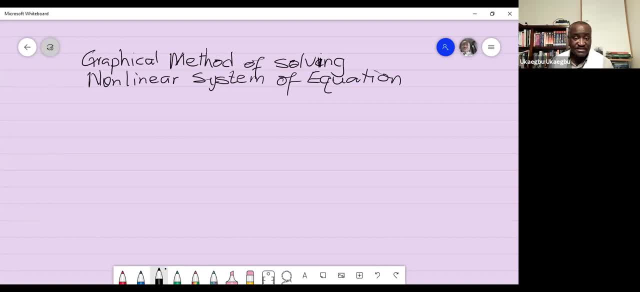 method, And then after we will look at game theory first, And then, after we will look at this, we will look at the other question. The question is: how do we solve the non-linear, involving non-linear systems of equation? One of it was substitution, So today we are going to 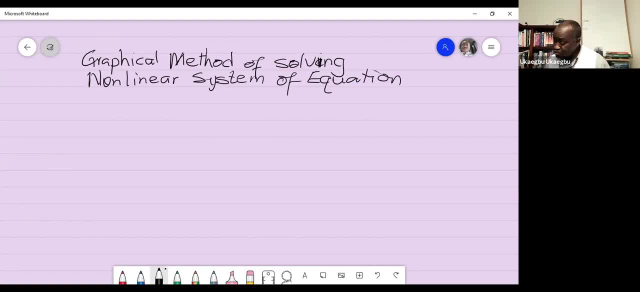 explore graphical method. All right, So now let's work with an example. Let's work with an example. All right, So example one. So the question usually go like this: Solve. See, this is very specific. Solve the equation using graphical method. So now, what's the equation that we need to solve? 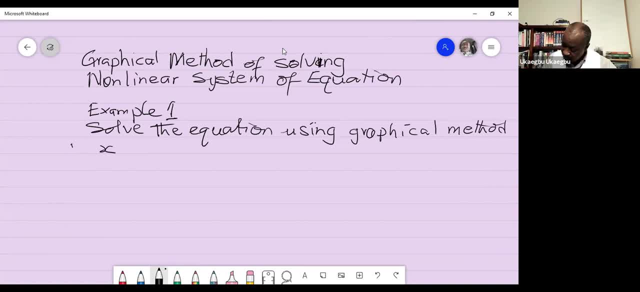 We need to solve x, y equal to x minus one and y equal to x squared minus x minus one, x squared minus x minus one. So these are the two equations that we need to solve And they say graphically: So once you have graphical method, so you have to create your, you generate your data set. 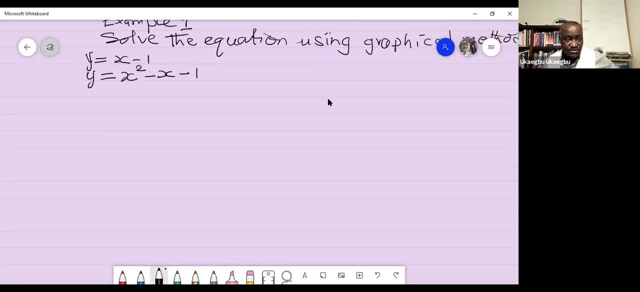 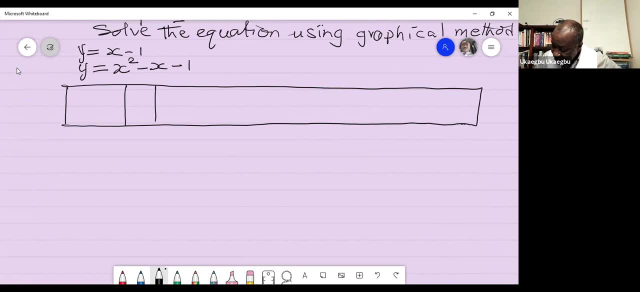 You have to generate your data set. So how do you do that? So you can draw your, draw, your, draw your table, And then, of course, you have your values for x and y. You have your values for x and then you generate the corresponding value for y. All right, So this is. 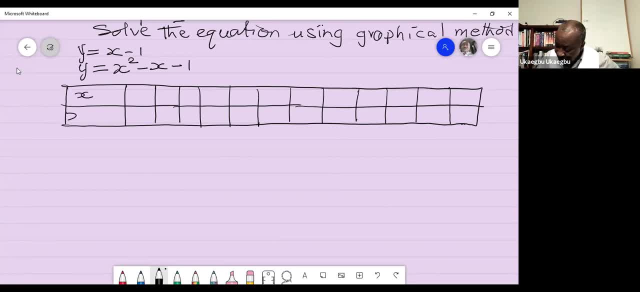 let's start our x here, And this is y equal to x minus one. So we can start with, for example, negative three, negative two, negative one, zero one, two, three, four, five, six. That should be. 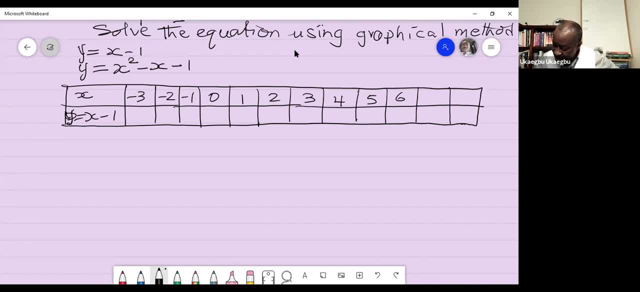 enough, And then we create the same thing for the other one. We create the same type of table for the second equation, So this is y equal to x minus one. And then we create the same type of table for the second equation, So this is y equal to x minus one. And then we create the same type of table for. 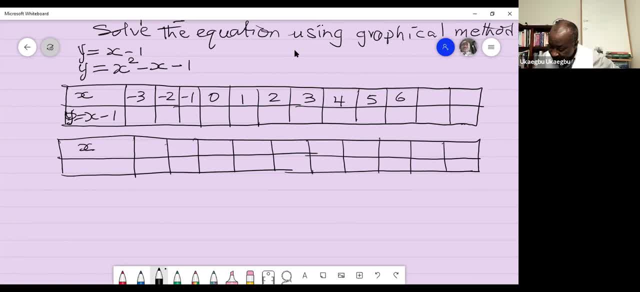 your x And this is your corresponding value of y. Y equal to x squared minus x minus one, And this is negative three. negative two. negative one. zero one. two, three, four, five, six, Okay, So next. 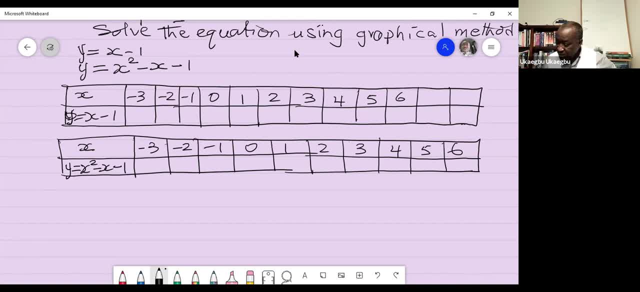 would be to generate your values for y. Okay, So now, how do you do that? So you have to generate your values for y. How do we do it? Can somebody give us a suggestion on how to generate the value for y? But let's start with the first one. So the first one. you plug in x and solve the equation. 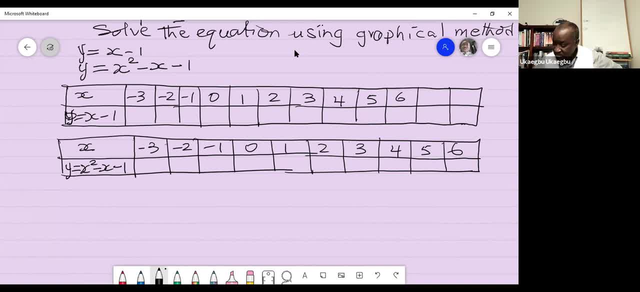 Okay. Who said So? plug in x All that time. Mention your first name, please, Javier. Okay, Javier, All right, Thank you. So what Javier said is for you to get the value of y, the corresponding value of y, you just have to plug in the value of y. 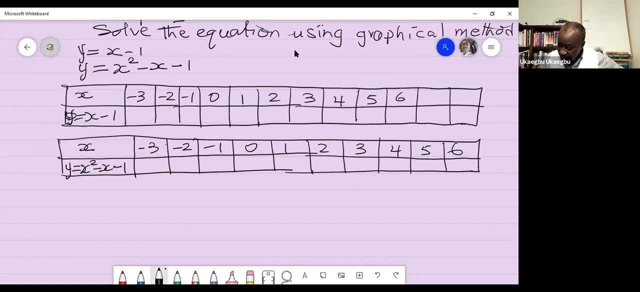 So let's try it for the first one. The first one is x, no y, equal to the first value. The first value is negative three. So all you do is you do negative three minus one, And that gives us negative three minus one. gives us what? Negative four? So you come here and write negative four. 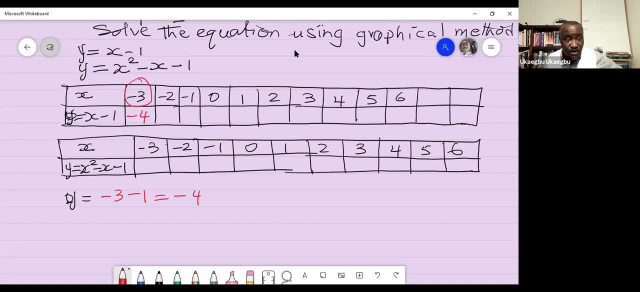 Okay, So let's do the same thing for the second one. The second equation is: y equal to negative three. whole squared minus bracket. negative three minus one. Did you see what I just did? So then this gives us negative three. is what Negative? 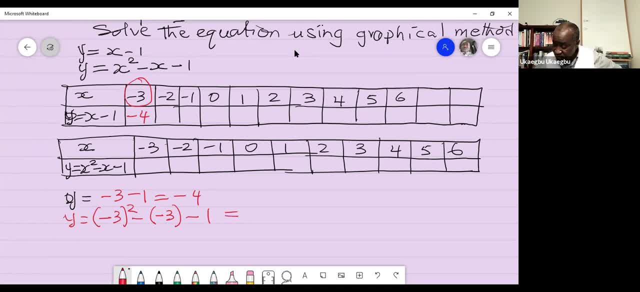 three squared is what Use your calculator: Nine, Nine, So nine, Then negative times. negative is positive, So you have plus three Minus one, So that should give us 12, minus one is 11.. So this gives us 11.. Positive 11. And you. 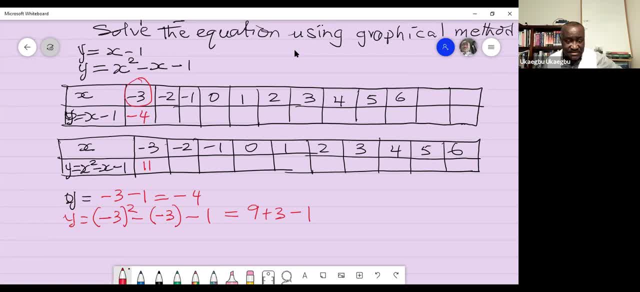 just repeat the process to create the data set. Speed it up, Use calculator. All right, So I'm going to give you two minutes for the first one and three minutes for the second one, A total of five minutes for you to fill in the gap. Five minutes. 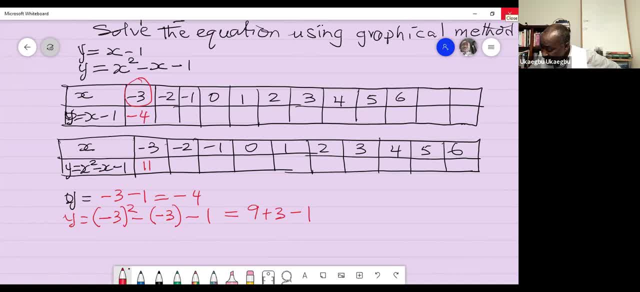 So you're working by yourself for five minutes And then, after five minutes, you are going to complete the table and then we start the process of plotting the graph. Okay, Everybody, five minutes passed right now, So I'm going to come back to you at 9.05.. Use calculator so that you make. 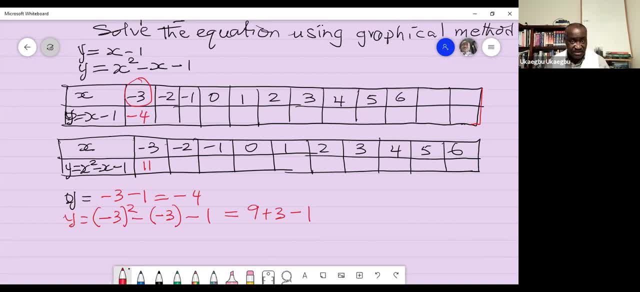 everything fast You can start. By the way, today's attendance is impressive. This is what we want Every day. we should be this number- Almost everybody- is here. I'm so glad You have two more minutes. If you have completed the first data, let me know. Just say yes. 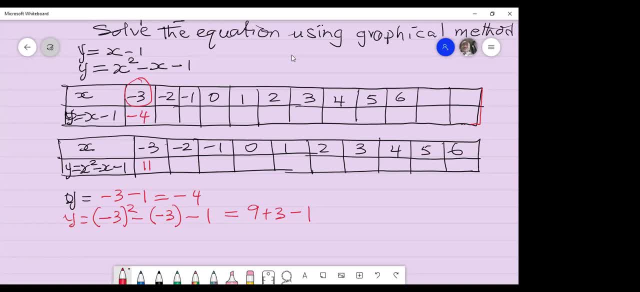 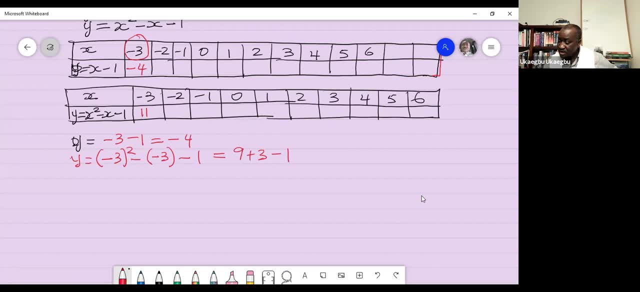 Yes, Yes, Okay, So okay, Let's move on. ladies and gentlemen, Let's move on. So I'm going to ask you to produce the numbers so that we can fill in the gap and then we take it from there. So I am going to be alternating. 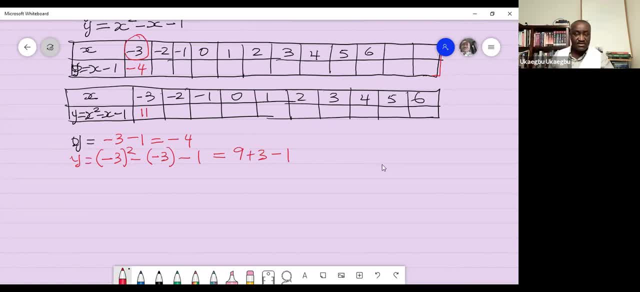 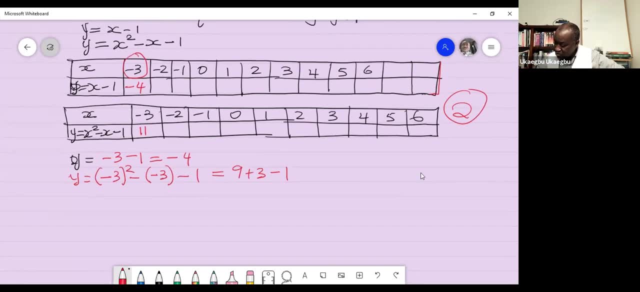 between the first data set and the second data set. For example, second data set, This is the second one And, of course, this is the first one. Okay, So on the first data set, what is the value of X? No, 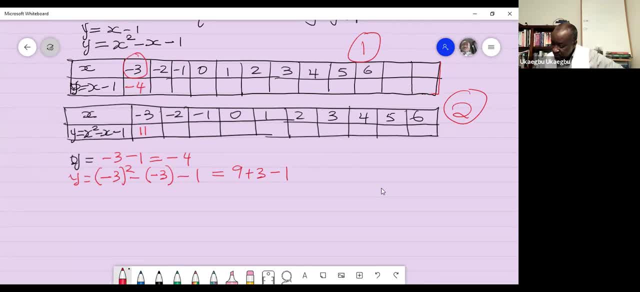 what is the value of Y when X is three? What is the value of Y when X is three? For the first one, First one. Do we all agree with that? So why no? Yes, Okay, So what that means is you're just solving Y equal to three minus one, which is two, So that's correct. 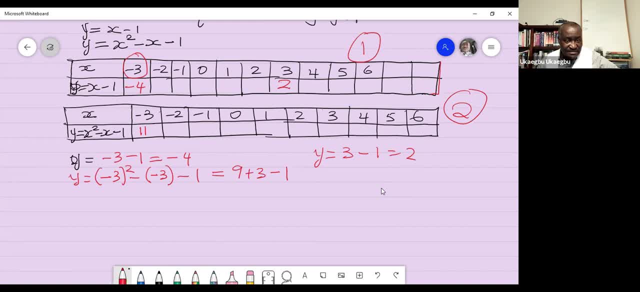 So what is the value of Y when X is zero? First one, Radha. Negative one, Negative one. Okay. What is the value of Y when X is six, Five, Five, Five? Okay, So we're done with that. So the second one. I'm going to focus everything on Y. 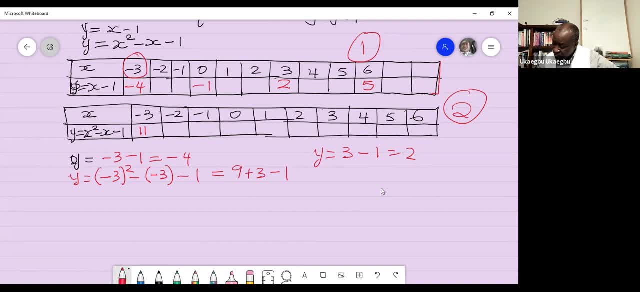 Okay, So I'm going to focus everything on second one now. What is the value of Y when X is zero? When X is zero, Is it negative one? It looks correct. So what you are solving is Y equal to zero, squared minus zero minus one. 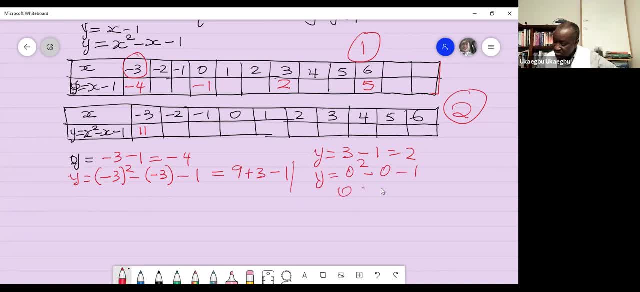 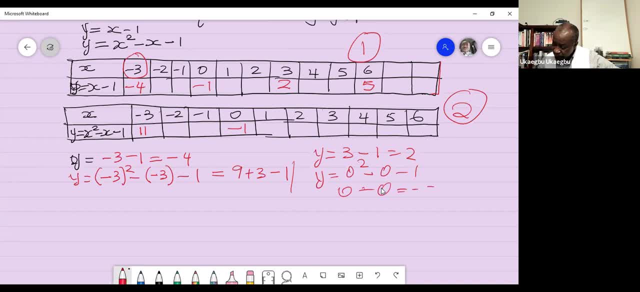 Okay, how about the value of y when x is negative 1? 1.. Okay, somebody said 1.. So let's check it out. You have, when x is negative 1, you have negative y equal to negative 1, whole squared minus bracket: negative 1 plus no, not plus minus 1.. 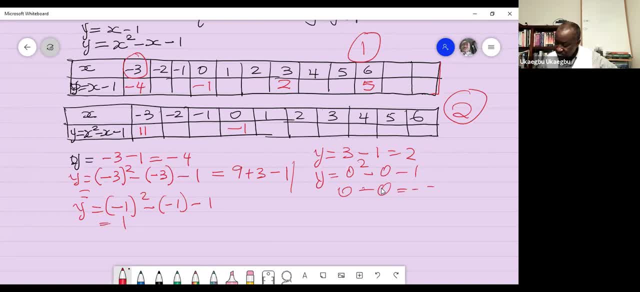 So negative 1, whole squared is 1.. Negative times negative is positive, So you have plus 1.. So 1 plus 1 is 1 minus 1.. So no, I'm sorry, 1 plus 1 is 2, minus 1 is 1.. 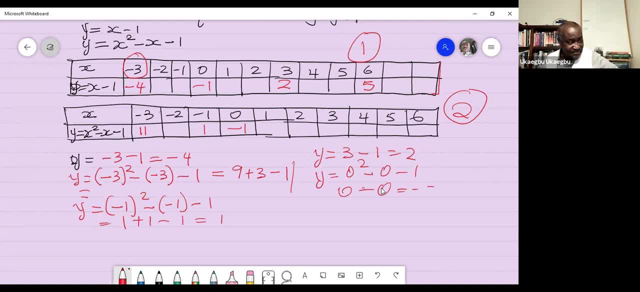 So this should be: 1.. Is that what you said? ranking: Yes, Okay, good. So now what is the value of y when x is 3?? 5., 5. Do we all agree with that? I got 2.. 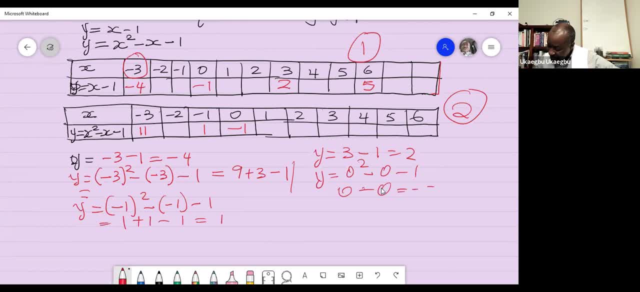 Okay, so let's verify it. Guess what you do. y equal to 3 squared minus 3 minus 1.. Remember: your equation is y equal to x squared minus x minus 1.. All right, So you should only worry about putting a parenthesis if the value is negative. 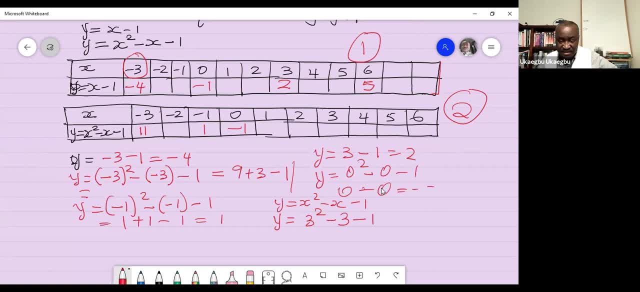 If the value is positive, just go ahead and plug it in like that. So now, 3 squared is 9.. 9 minus 3 is 6.. So this is 9 minus 3 minus 1, which is 5.. 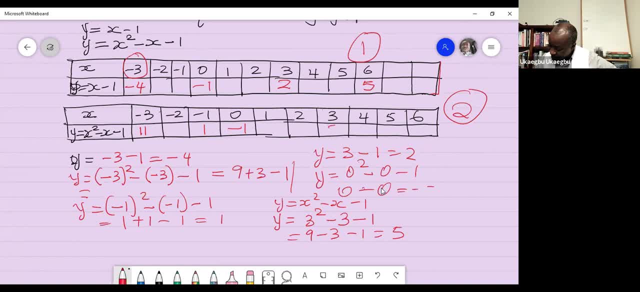 It is 5.. What were we solving? So? this is 5.. Okay, So now, once again, let me demo how to do this using a calculator. Let me demo, show you What you are doing. is you open a parenthesis? 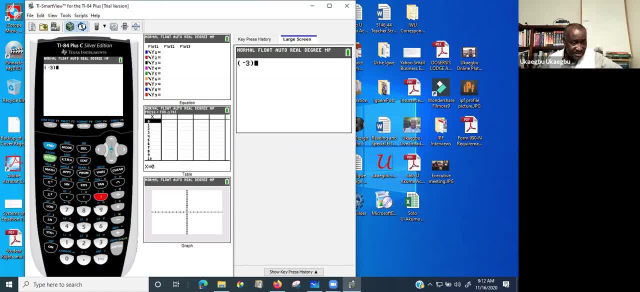 You say negative, You close the parenthesis. Then you do square, You do square So, and then, once you do square, then you say minus, your regular minus. You open up a parenthesis. You also say negative: 3. You close your parenthesis. 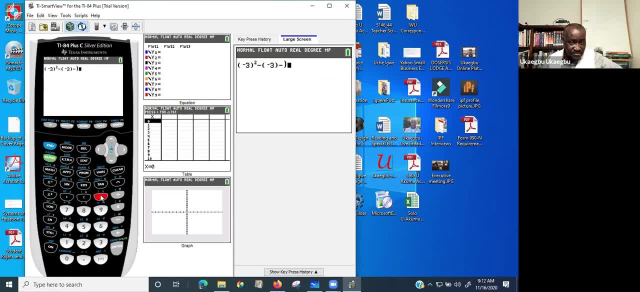 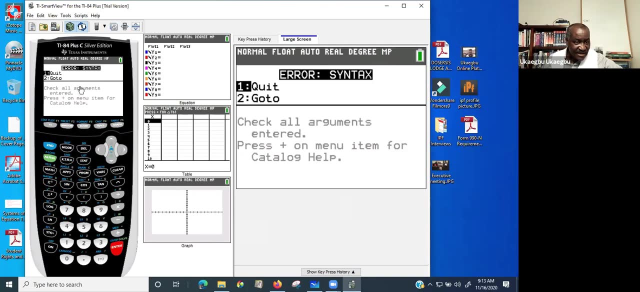 And then you type negative 1.. Is that correct? And then you hit your enter key, Boom What It says: error. You put a parenthesis instead of a negative 1.. Oh, I'm sorry, So I need to go back. 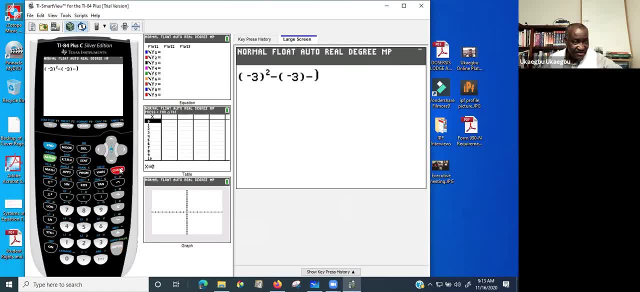 Okay, So let me start all over. I'm sorry. Thank you for observing the error. Oh, you are right, You are right, You are right. So let me repeat, Thank you. Negative Black parenthesis: Negative 3.. 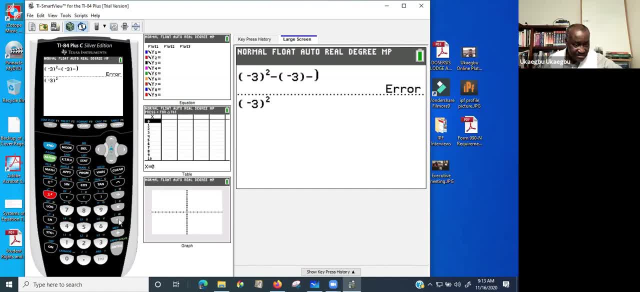 Then close your parenthesis Squared Minus. Open parenthesis Negative: 3. Close your parenthesis And then you say minus again, And it should be minus 1.. Right, Okay, I guess this is correct now. Okay, You see, it gave us what we got manually. 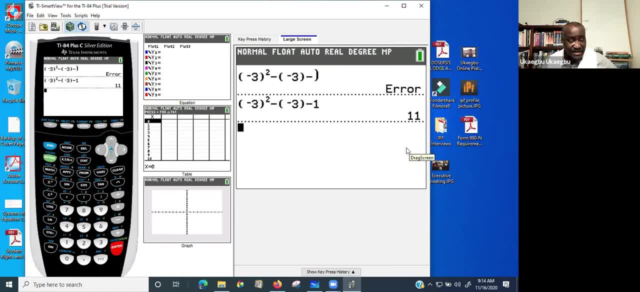 So that's how to do it, ladies and gentlemen. So, now that we have generated our data, we are going to plot the graph, So I will go back to the screen. So Now, please pull out your graph paper. You can use your graph paper. 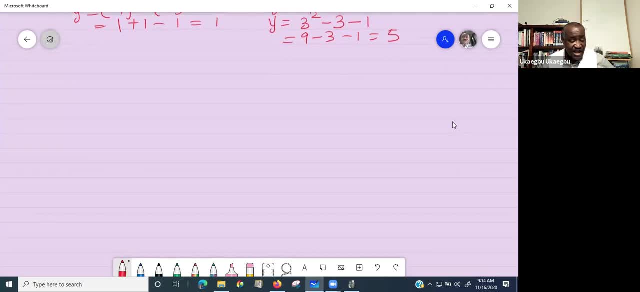 If you don't have a graph paper, here's what you do. If you do not have a graph paper, here's what you do: Use your regular line paper And then get a straight edge and create a graph paper for yourself. So how do you do that? 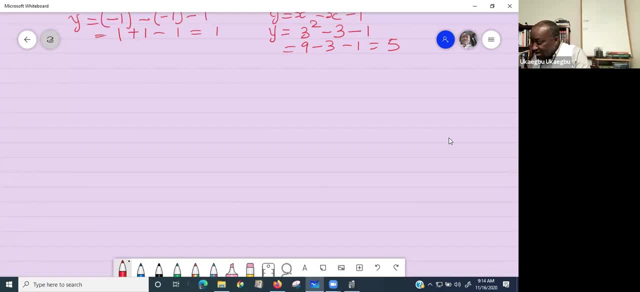 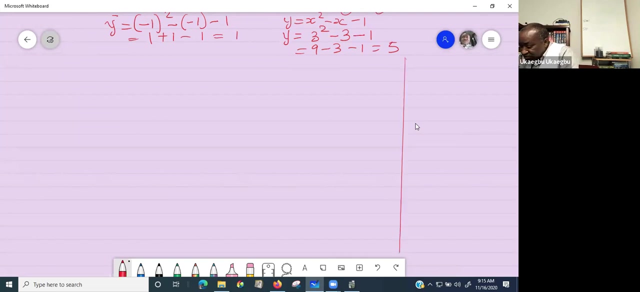 Just place a ruler on your regular graph paper. Place a ruler right there And do the following. Here's what I'm about to do: Just draw a set Of vertical lines. So draw a set of vertical lines. I hope you're seeing the screen. 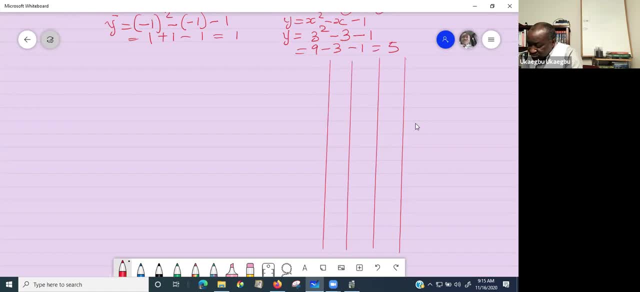 So draw a set of vertical lines, Just do an approximate, you know, spread it evenly. What you're doing now is approximation. I mean, if you have the time you can measure them, but that's not necessary, Okay, So I just created a graph. 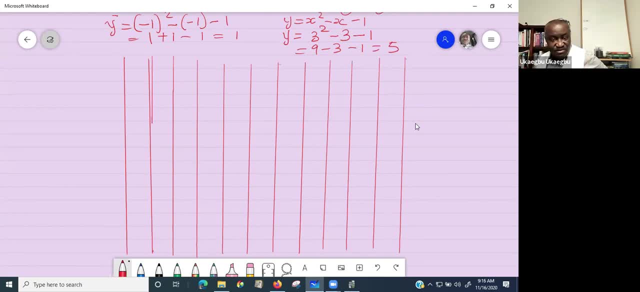 The horizontal line is my horizontal line, The vertical line is the one I just drew. So now, what do you do next? So now, let's draw the real graph. Let's draw the real graph. Um, just draw your, draw your horizontal line and then pick one point and draw your vertical line to represent your X and Y, to represent your X and Y. 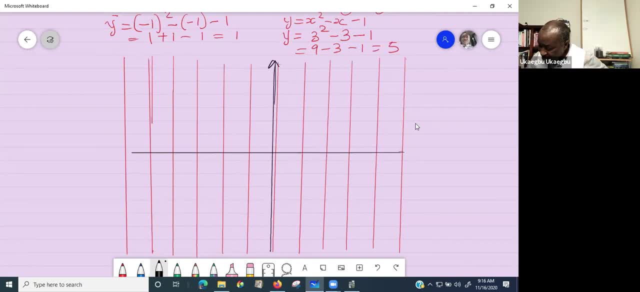 Okay, so that's your X and Y. This is your Y axis and this is your X axis. Of course, you can always extend your line. So, uh, this is uh. one, two, three, four, five. 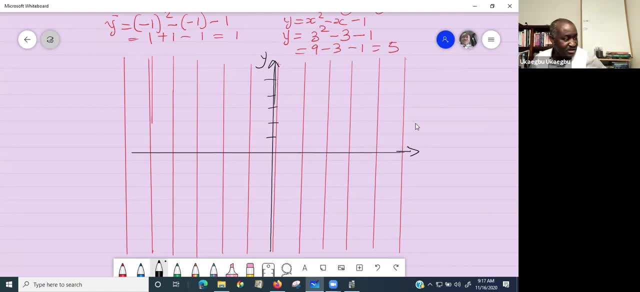 It can also be two, four, five, six, seven, Uh, maybe we actually need to do two. So this is uh, two, four, six, eight, 12.. So, uh, the highest value for Y, uh, for X, is six. 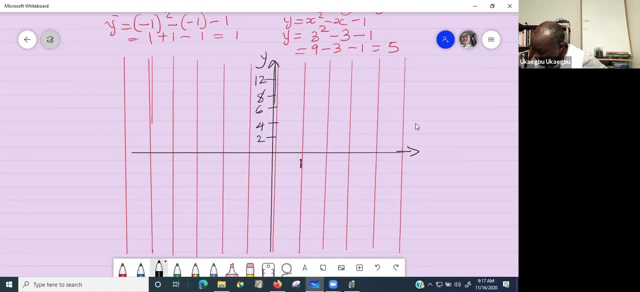 So we can have six values here: Uh, one, two, three, four, five. uh, six is somewhere here, Six, seven, And the same thing goes here. So this is your zero negative, one negative, two negative, three negative, four negative, five negative, uh, six. 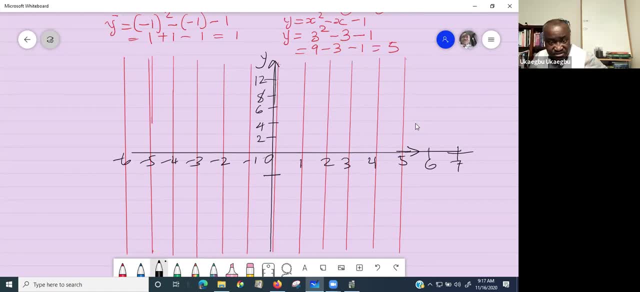 And you have your. the Y value scale is supposed to be even So, uh, the same scale, the the upper side and the lower side. So you have two, four, six, eight, 10.. Uh, this should actually be 10 here. 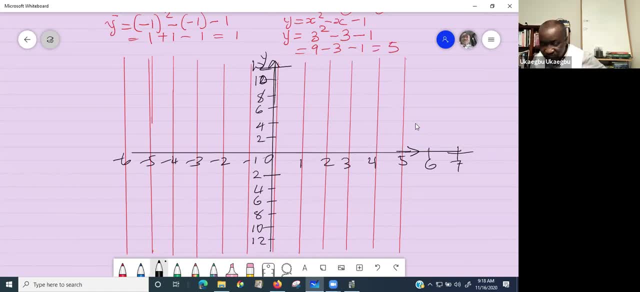 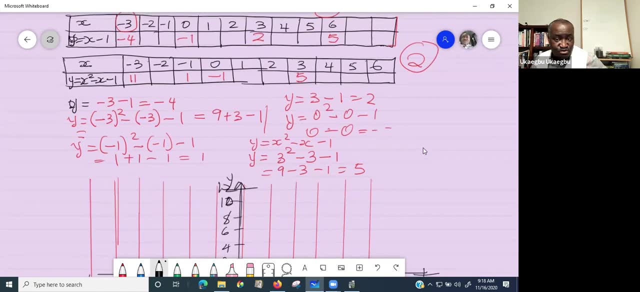 And the next one, 12., And then 12.. So let's start with the first. Let's start with the uh, you can start with any of them, but you are going to plot the two graphs in one scale. You are going to plot the two graphs in one scale. 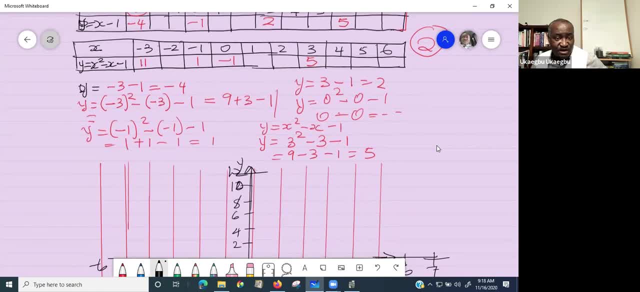 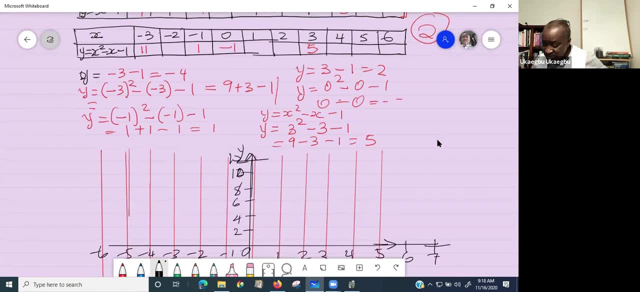 So let me use, let me plot the second one and then you plot the first one. Okay, So I'm going to plot the second one. So when Y is, when X is three, Y is 11.. When X is three, which is here, 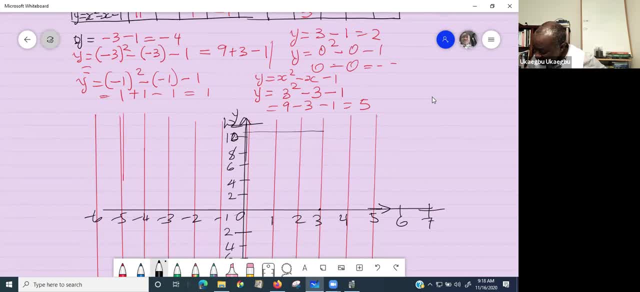 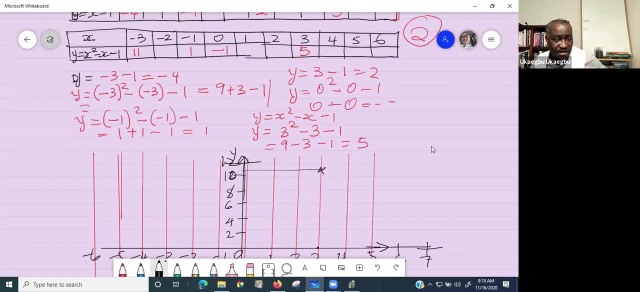 Why is 11?? 11 is somewhere here, So this is your first point. Next, When: when X is negative one, Y is one. When X is negative, one X is. I'm sorry, I made a mistake. I'm sorry. 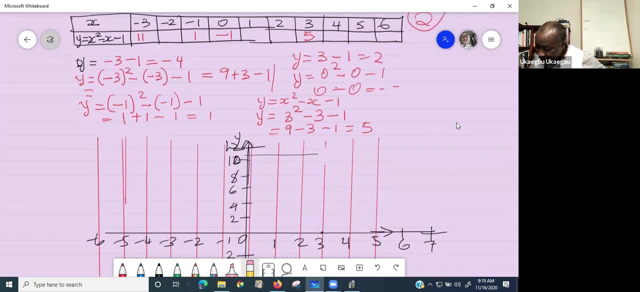 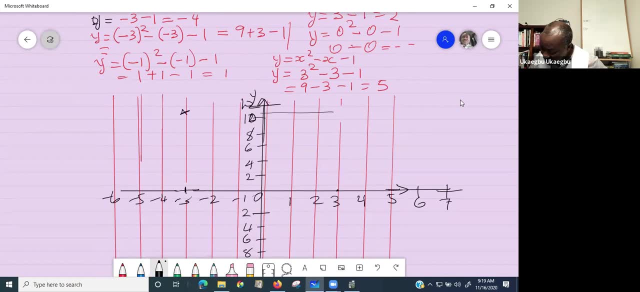 There's the mistake When, when X is negative three, Y is 11.. So this is negative three, negative three, here, 11.. So that 11 is supposed to be here Now when X is negative two. what is the value of Y when X is negative two? 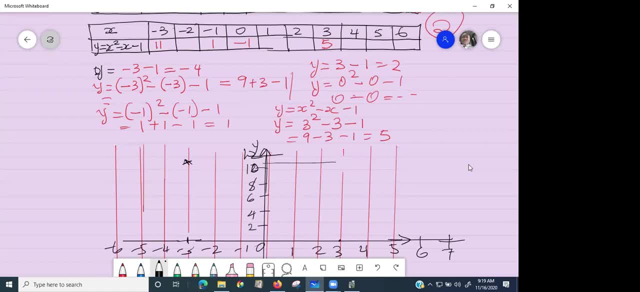 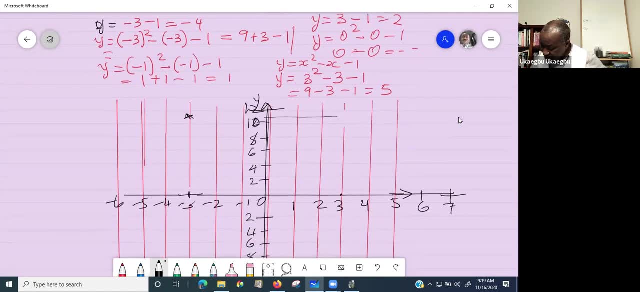 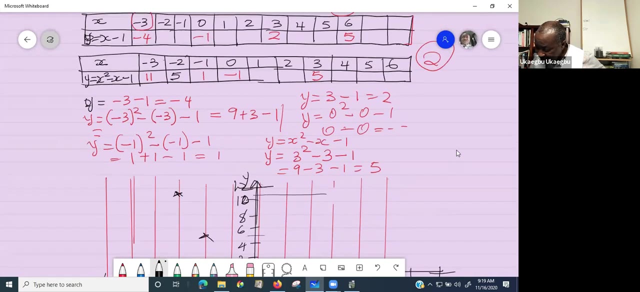 Look at the table you generated. is it? is it what? five? five. Okay, So when X is negative two, Y is five according to the result he gave us. So this is five here. Negative two is somewhere here. Then when X is negative one, Y is one negative one. 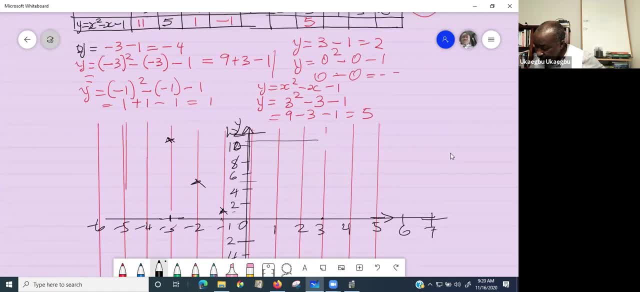 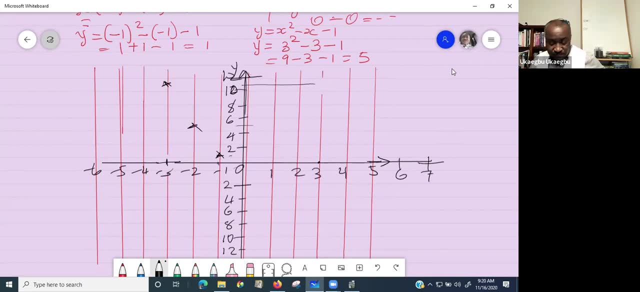 One is somewhere here. When X is zero, Y is what? Negative one. When X is zero, Why is Negative? uh, negative one? No, I'm sorry, When X is zero, Y is negative one. Negative one is somewhere here, somewhere here. 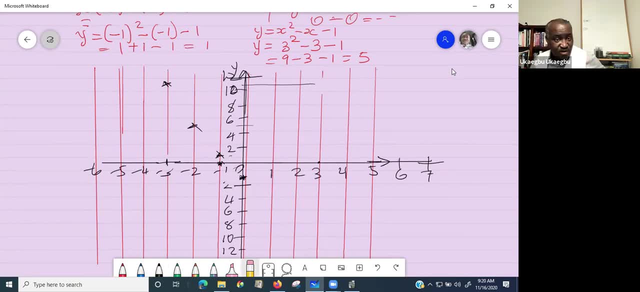 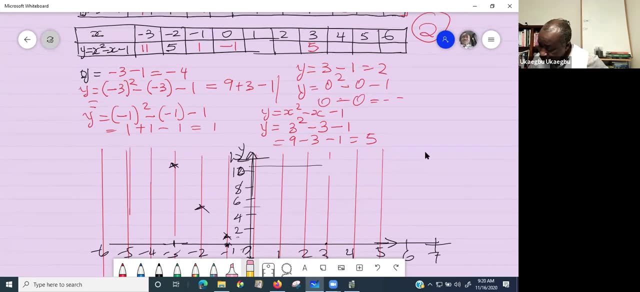 Negative one. All right. Then next is: when X is what Next value? please help. When X is one, what is Y? when X is one, What is Y? who did it? The second one? Yeah, When X is one, what is Y? 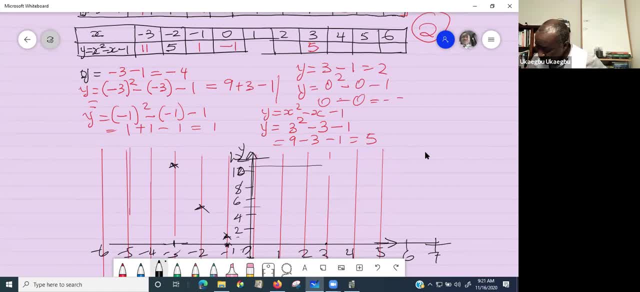 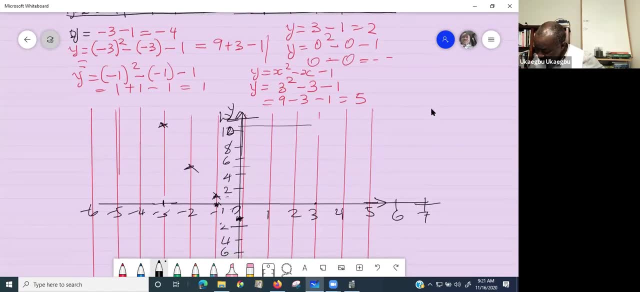 I think I think I got it Negative one. Is it negative one as well? Okay, Let's use negative one. Okay, When X is one, Y is negative one. So this is one. negative one is somewhere here. Let's go. 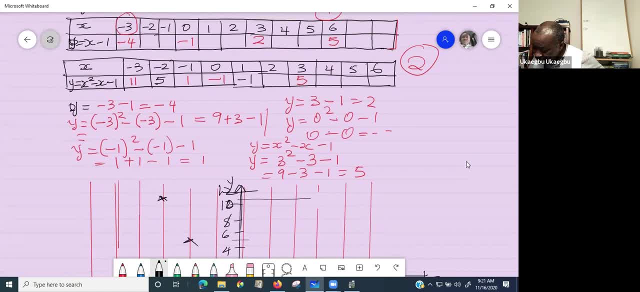 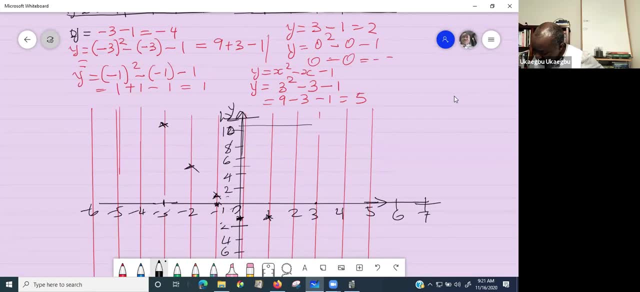 What next When X is um two? what is Y one, one? Okay, When X is two, are you sure it is one? Let's do that. one again When X is two. So you are using both tables. 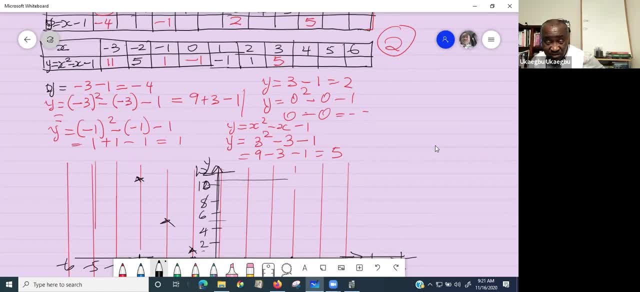 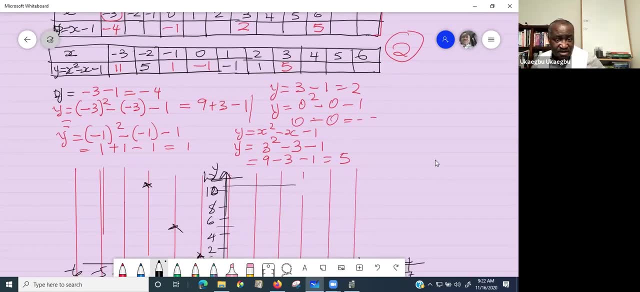 Now I'm using the second one, I'm plotting the second one. Um, you are going to plot the first one, I'm plotting the second one, So let's do. Oh, I'm sorry. When X is two, when X is two, Y is one. 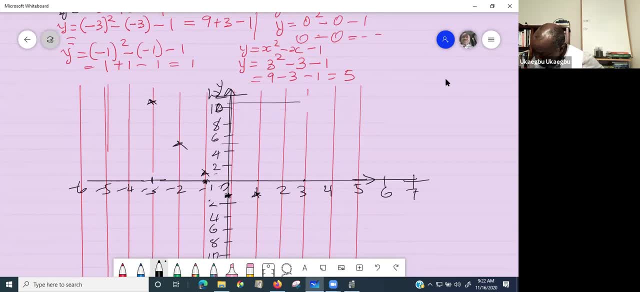 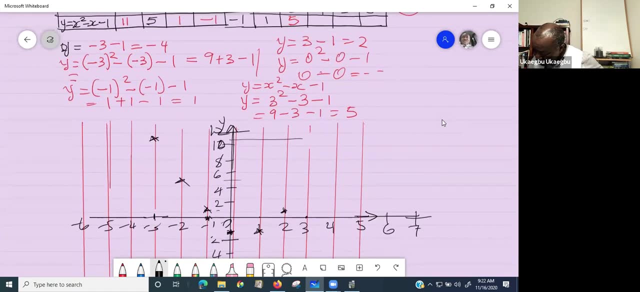 All right, let's go. When X is two, Y is one, So Y is somewhere here. When X is three, Y is what Five? X is three, Y is five, Five. This is four. Five is somewhere here. 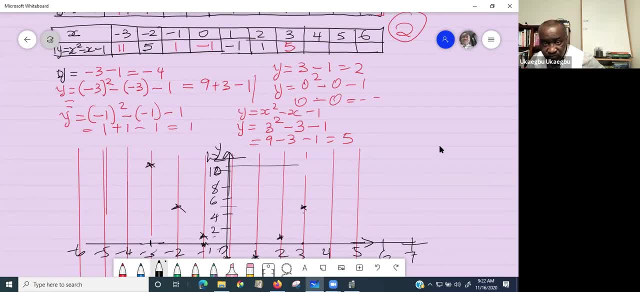 When X is um four, what is Y? When X is four, what is Y? I got 11.. You got 11.. Let me write 11.. So when X is four, Y is 11.. So you have somewhere here. 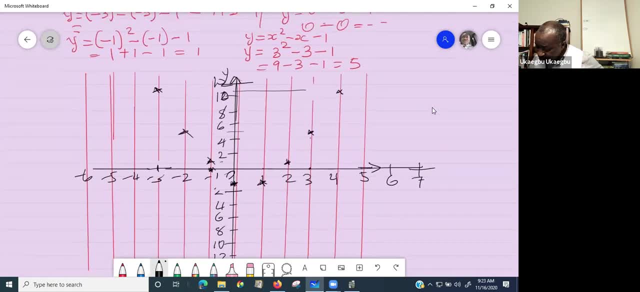 Now you see, your graph is a parabola, So you just joined the point, So I'm going to join the point. Then, at this point, you have a call, a smooth call. This is a call, This is not a U. 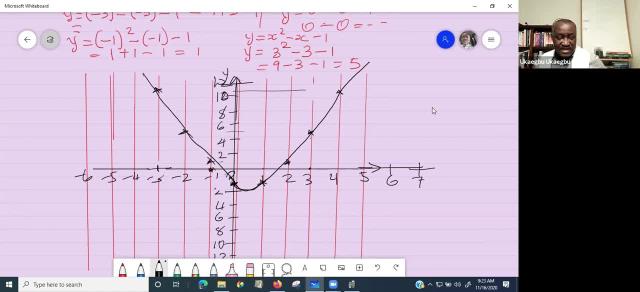 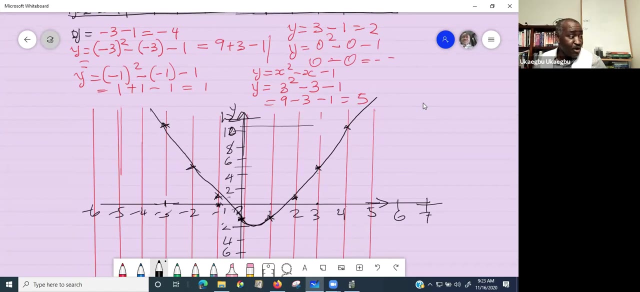 You know. all right, so this is basically how the graph for- uh, the second one looks like. So I want you to plot the graph for the first one, plot it on the same scale and then note the point of intersection. So once you plot it, it's going to give you a straight line, and then join your point. 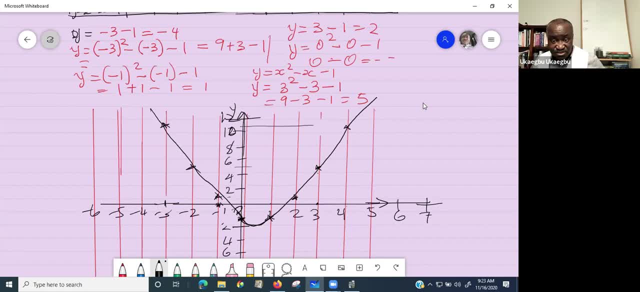 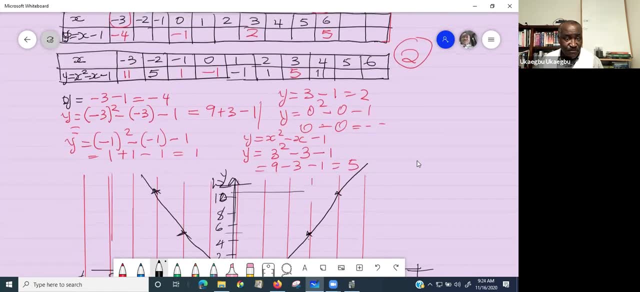 And then, once you join your point and note the point of intersection, All right, So I'm going to give you how many? I'll give you three minutes, So plot the second one. That means you must have completed the data for the second one. 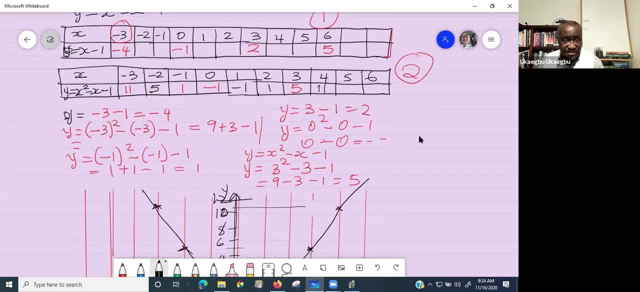 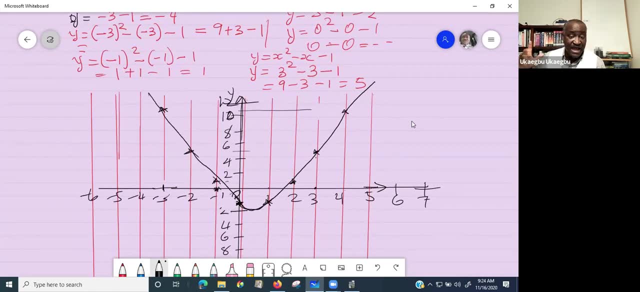 And no, I'm sorry, The first one. plot the first one and then note the point of intersection with the graph of the second one. So I'm going to give you five minutes, please Not five. three, three, three, three, three, three. 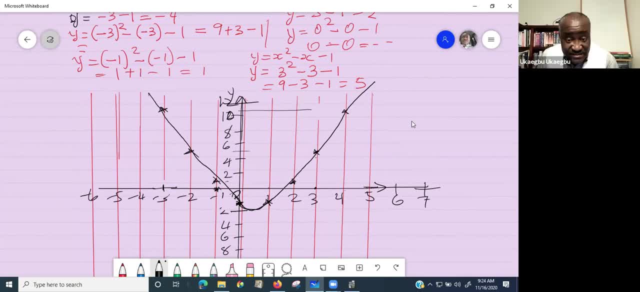 You want us to plot it on the same graph, Exactly The same place. Do not create any other scale. Plot it at the same scale, the same coordinate, the same everything. Okay, Once you are done, note the point of intersection. 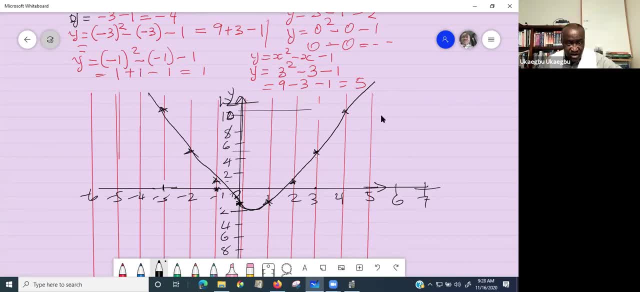 So that's what I'm going to ask you. Okay, Three minutes is gone. How many people have finished plotting the first one? Say yes. if you did, Yes, Yes, Okay. So what are the points of intersection? Did you draw the line? 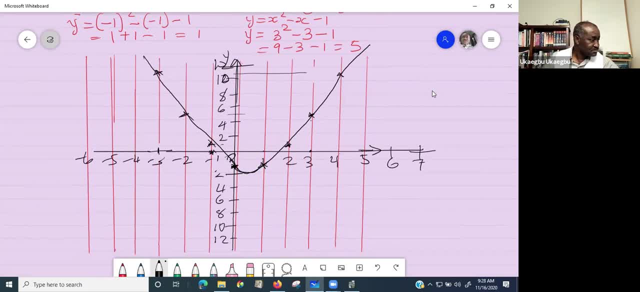 So what are the points of intersection? I got zero negative one and two one. You have to get just Just one. No, no, no, no, no. The first point of intersection is: what, Please? Zero negative one. 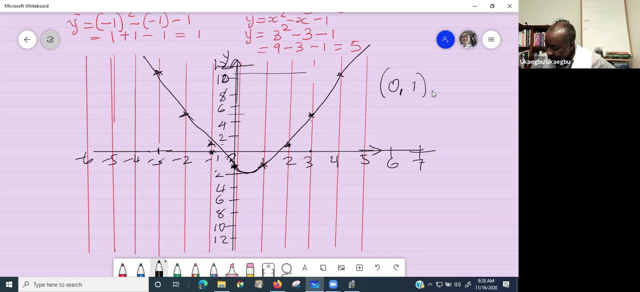 Okay, Zero negative one. And then the second point of intersection is what Two one Who said so, Gabriel? Okay, Thank you, And that's correct, That's correct, All right, So that's correct. So that's how you graph an equation- nonlinear equation- graphically. 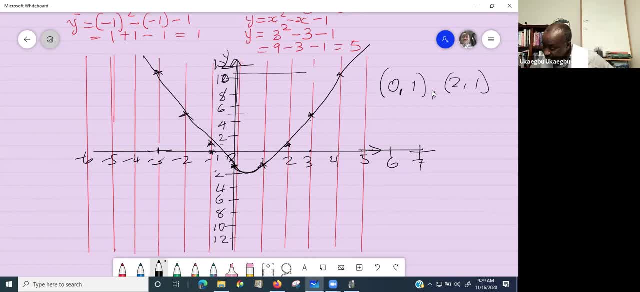 So, from what she said, the points of intersection are going to be zero and negative one. Zero is X- and negative one. Put this right here Here, Let me put it right here. And then two and negative, and one, Two and one. 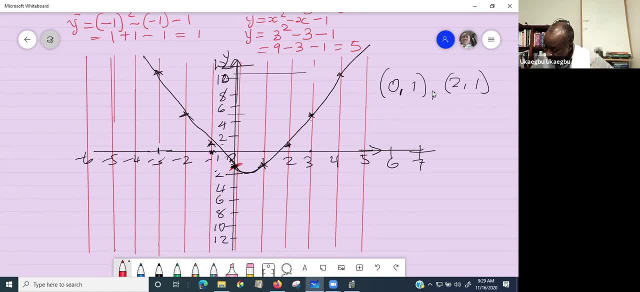 Two and one is two and one Somewhere here. So you draw your own line that cuts across that point And that's your solution. So here is two comma one And here is- I mean I want to put it down here. 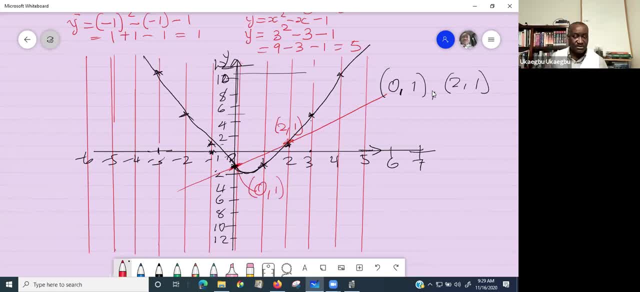 Zero, comma one, And that's your solution And you are done All right. So if for any reason, if you did everything right and you don't have a point of intersection, what that means is that the equation does not have real solution. 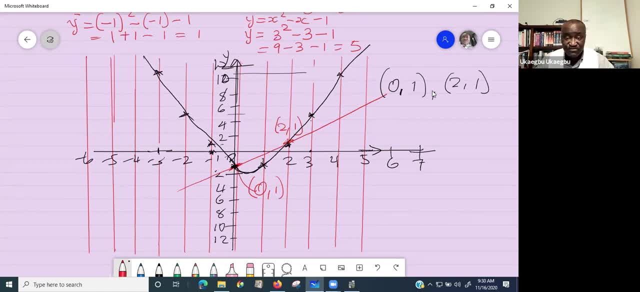 Let me repeat. Let me repeat: If you, after getting all your data values correctly, and you have plotted correctly, and there is no point of intersection, what that means is that the equation do not have real solution. That's what it means, As as soon as it has points of intersection, those points of intersection is your solution. 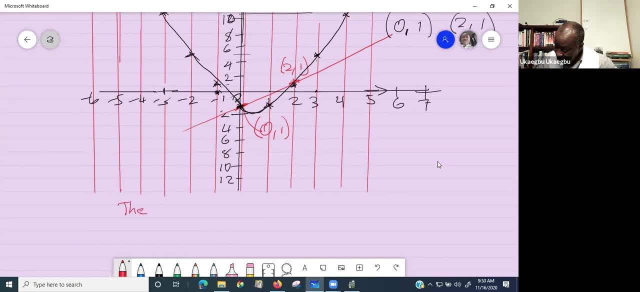 So you can definitely say: the solution of the given equations is zero. That's what it means: 0, 1, and 2, 1.. That's it And you're done All right. So right now the time is 9.30. 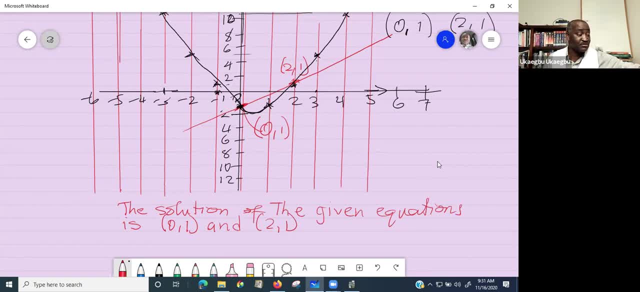 I'm going to give you one more graph to do This you are going to do completely by yourself And you have to finish by the end of the class period. You have about 25 minutes to do one, So I'm just going to give you one. 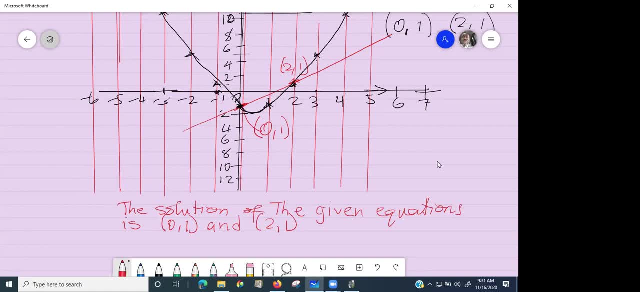 Mr O'Keefe, Yes, Is it 0, negative 1 or 0, positive 1?? It is 0, negative 1.. Sorry, It is 0, negative 1.. That's what this thing here is. 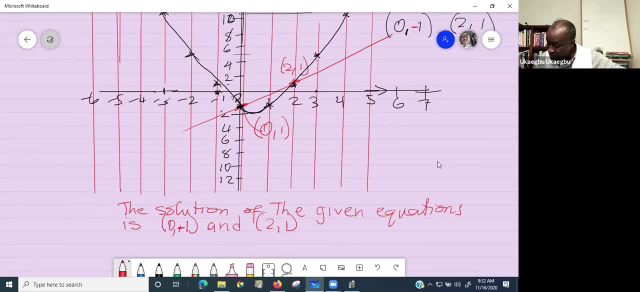 It is 0, negative 1.. Gabriel, I hope you got negative 1.. OK, It's 0, negative 1.. You see, You can actually see it from the graph. Here is negative 1.. Positive is on top. 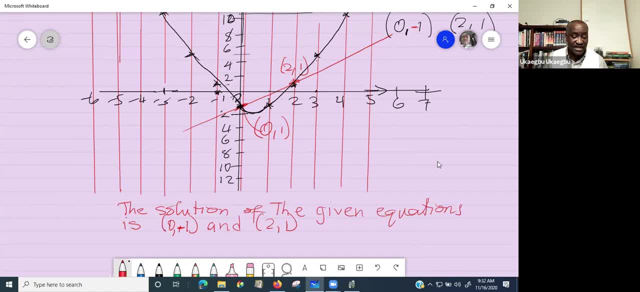 We didn't even have a value on the positive side, So it is 0, negative 1.. All right, Now here's the task. I don't want to waste Much of your time Again. you have 25 minutes. 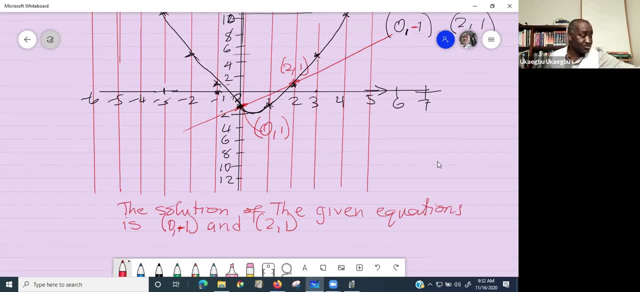 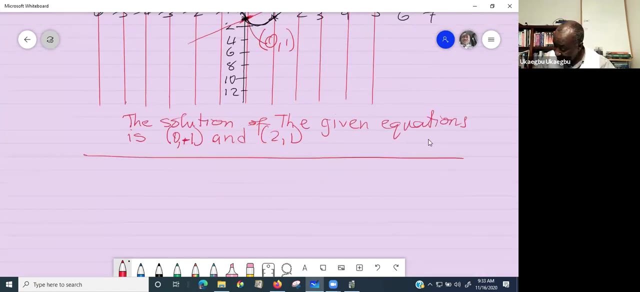 So just use graphical method to solve the following system of equations. Use graphical method. So now let me give you the equation to solve. This is going to be super easy, So let me. You are going to finish at the end of the class period. 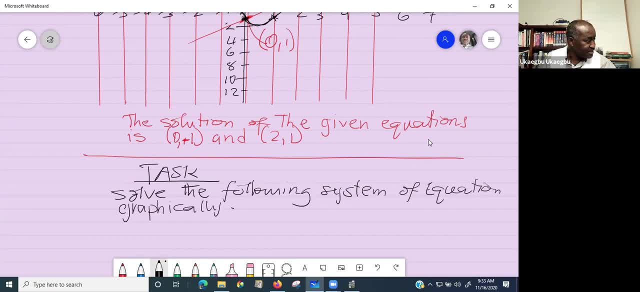 And the task is solve. So it is your system of equations. You are going to solve this. Why? Now? I'm going to give you the will to solve. The first is the you. So we, we need to keep it simple.